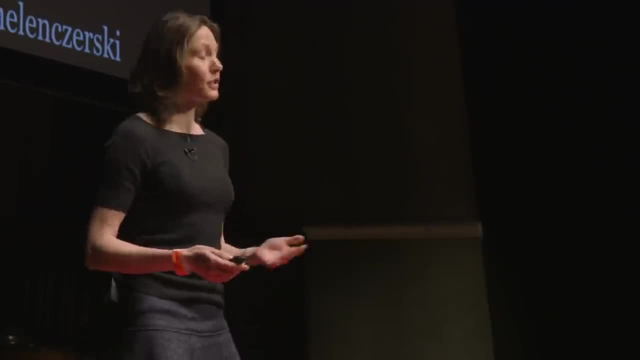 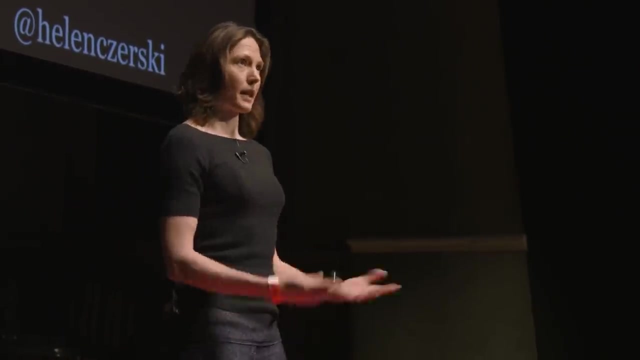 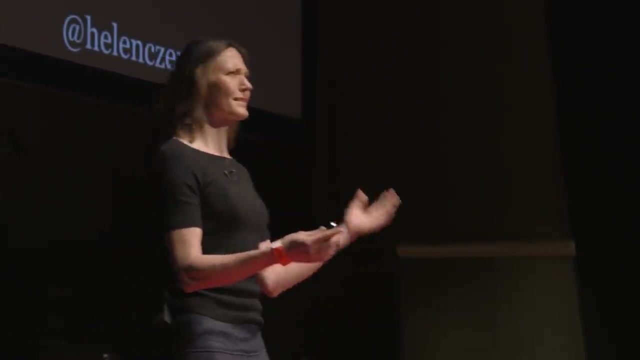 let's be honest, And nana came along and she looked at this folder and she said what's that? And I said it's quantum mechanics. nana And I tried to explain something about this. what was on the page? It was to do with the nucleus and Einstein A and B coefficients. 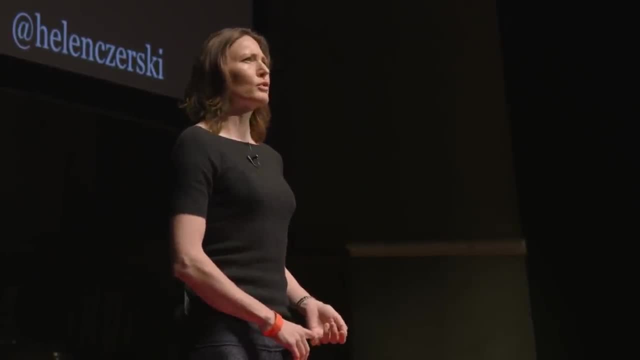 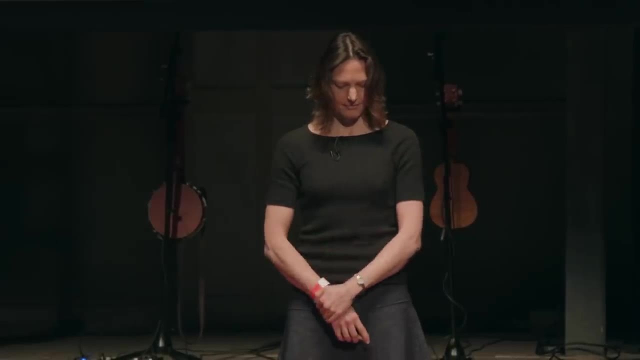 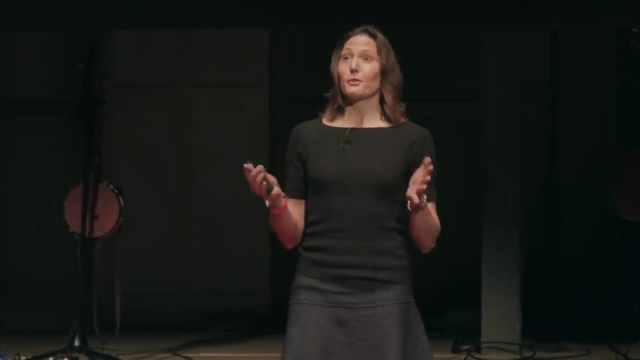 And nana looked very impressed And then she said: oh, what can you do when you know that? Don't know, nana, And I think I said something about computers Because it was all I could think of at the time. But you can broaden that question out because it's 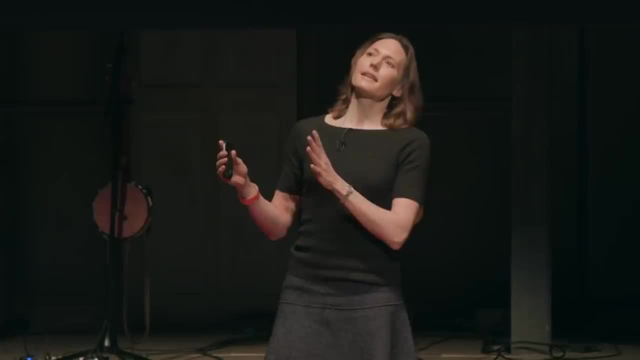 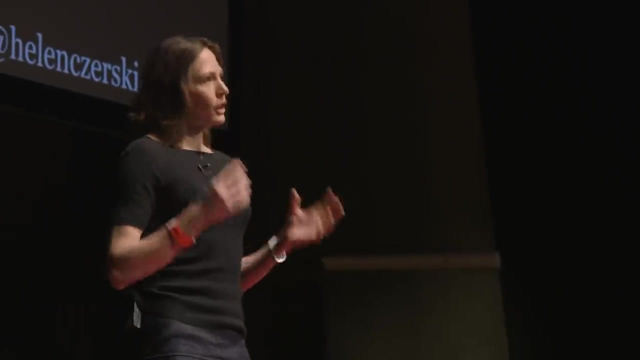 a very good question: What can you do when you know that? when that is physics- And I've come to realise that when we talk about physics and society and our sort of image of it, we don't include the things that we can do when we know that Our perception of what physics is. 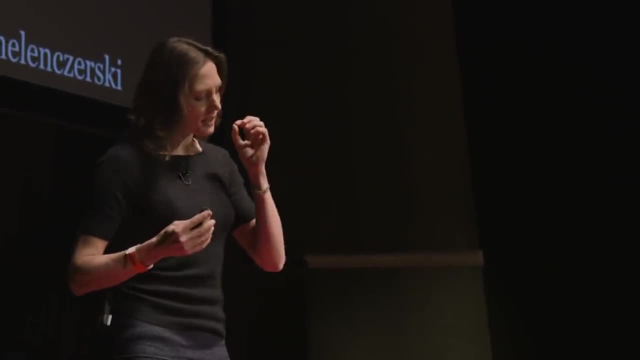 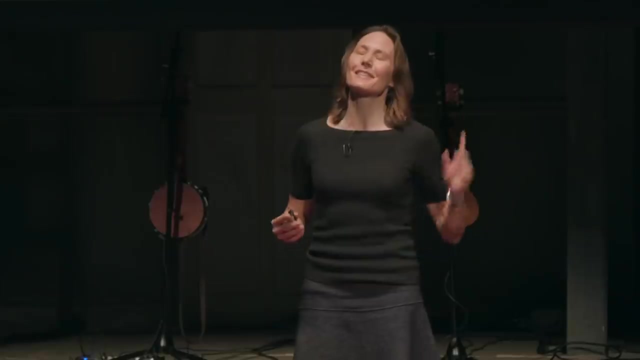 needs a bit of a shift. And not only does it need a bit of a shift, but this perspective, sharing this different perspective, matters for our society, And I'm not just saying that because I'm a physicist and I'm biased, And I think we're the most important people in the world. 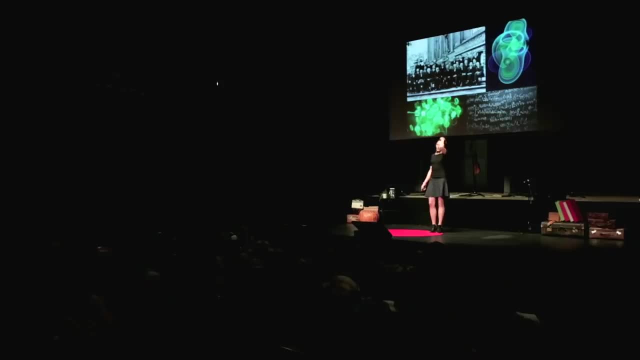 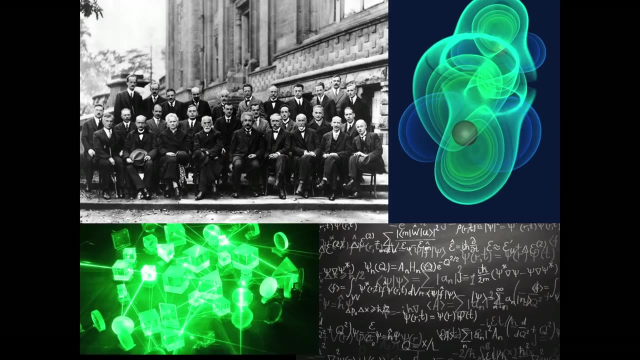 Honest. So the image of physics right. We've got an image problem. let's be honest, It hasn't moved on much from this. This is a very famous photograph. It's from the Solvay conference in 1927. And this is when the great minds of physics were grappling with the nature. 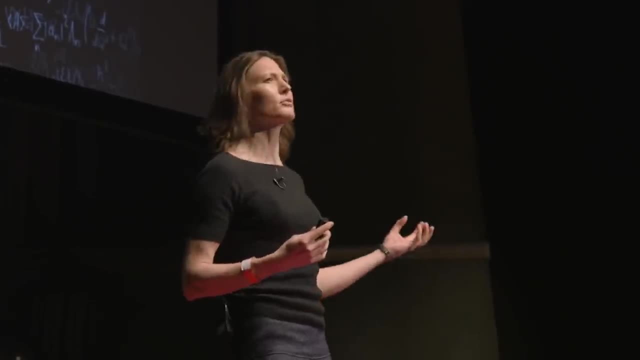 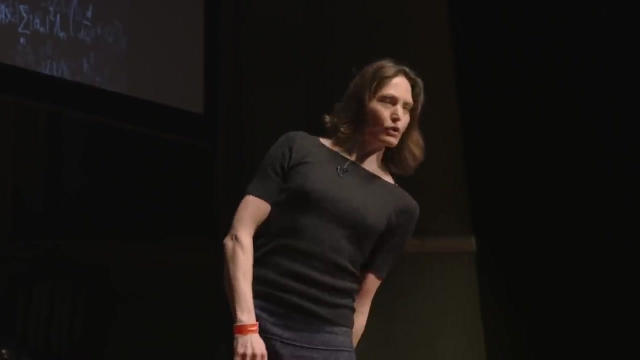 of determinism and what it means only to have a probability that a particle might be somewhere and whether any of it was real. And it was all very difficult And you'll notice that they're all very stern-looking men in suits, Marie Curie, I keep nearly saying Marie Antoinette, Which would 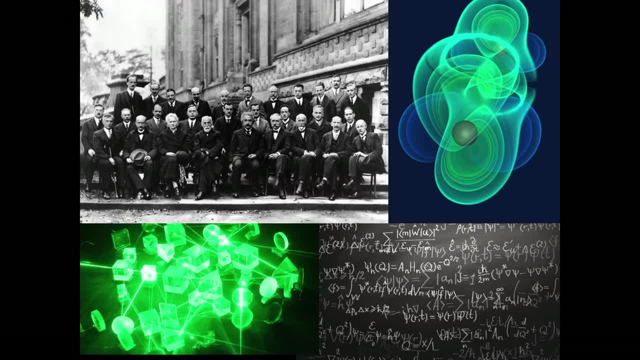 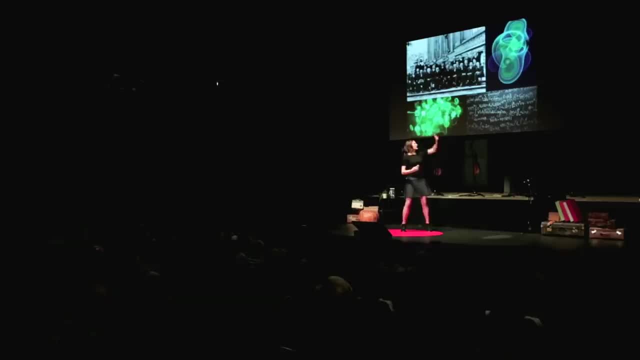 be a turn-up for the books Marie Curie. third, from the left on the bottom. there She was allowed in, but she had to dress like everybody else. So this is what physics is like. There's all this kind of hieroglyphics. These are to do with waves and particles. That is an artist's impression of 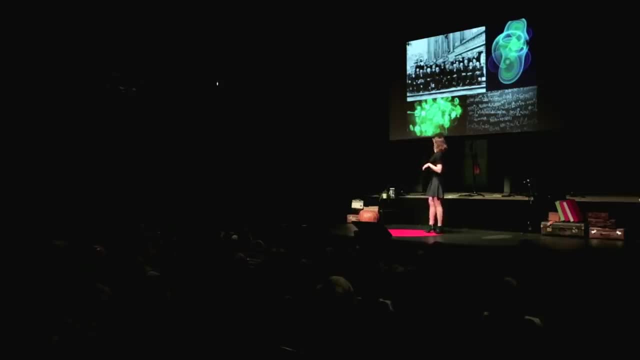 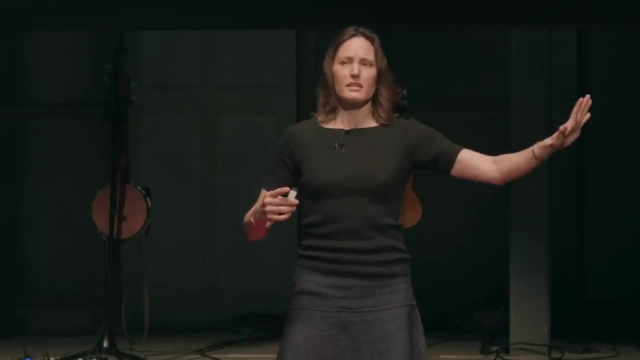 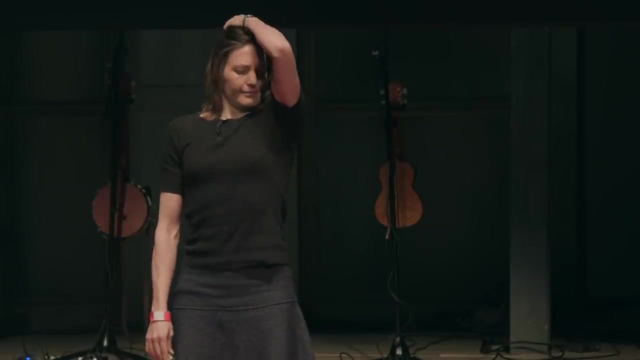 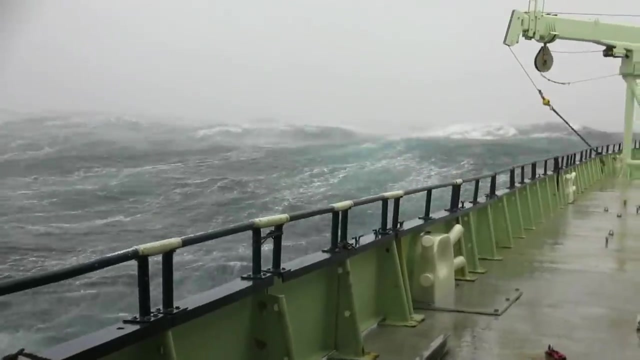 It's weird and difficult, It's done by slightly strange people dressed in a slightly strange way, It's inaccessible, It's somewhere else And, fundamentally, why should I care? And the problem with that is that I'm a physicist and I study this. This is my job, right? I study. 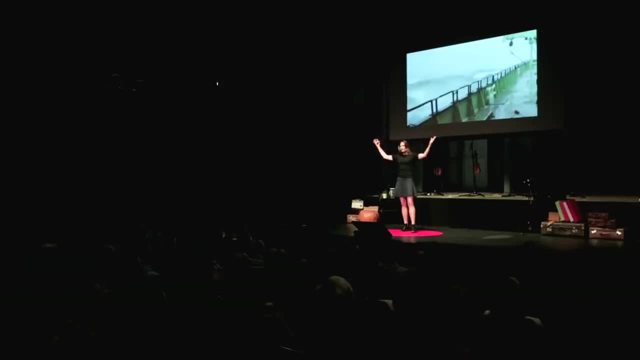 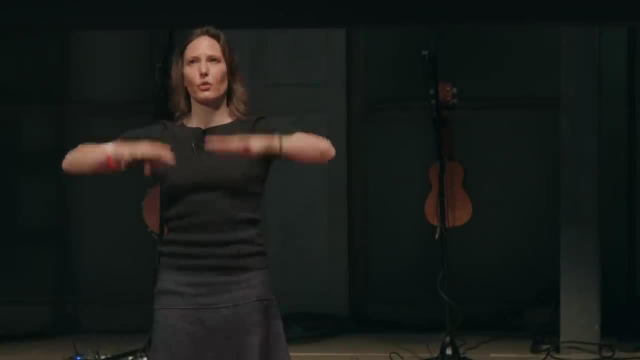 the interface between the atmosphere and the ocean. The atmosphere is massive, The ocean is massive. The thin layer that joins them together is really important because that's where things go, from one huge reservoir. You can see that- the sea surface. that was me who took this video. the average height of those. 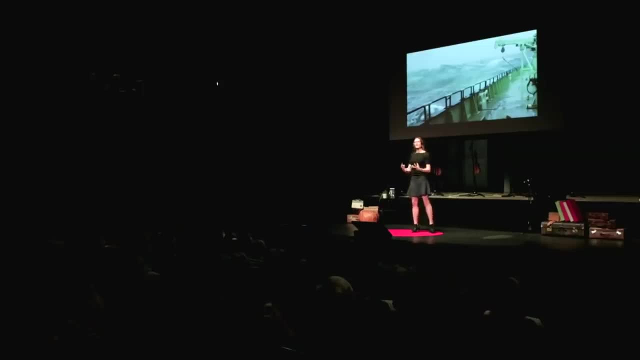 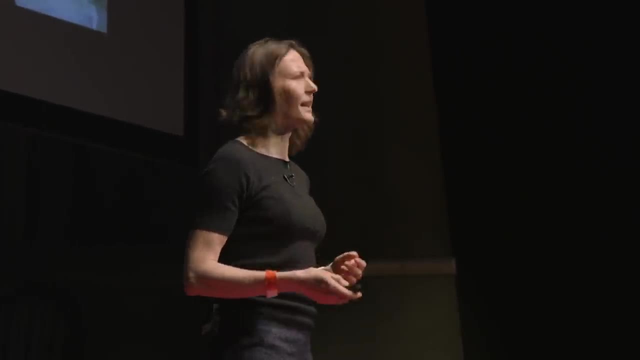 waves, by the way, was 10 metres. So this is definitely physics happening here. There's lots of things. This is definitely physics, And yet it's not included in our cultural perception of physics, And that bothers me. So what is included in our cultural perception of physics? Well, 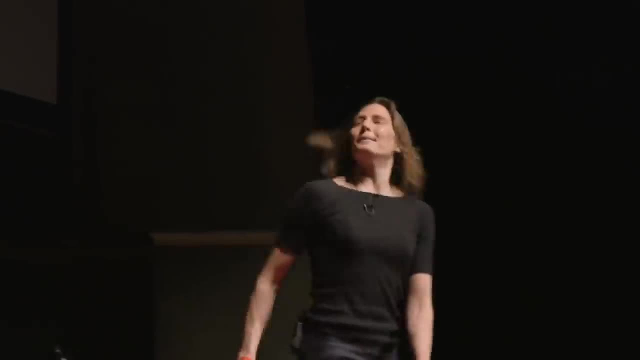 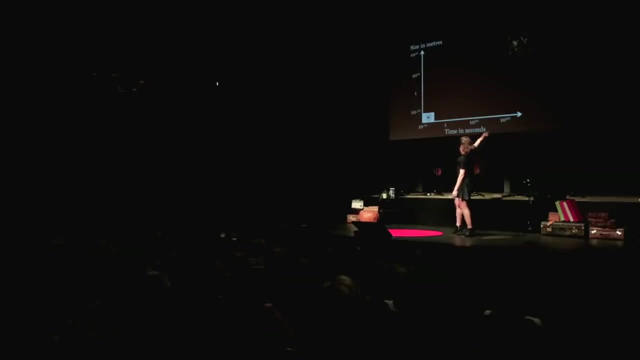 so because I'm a physicist, there has to be a graph, right, That's allowed. So we've got time along the bottom here from very small, very fast things. So we've got time along the bottom here. So we've got things there. It's very long things that take a long time over here. Small things at the 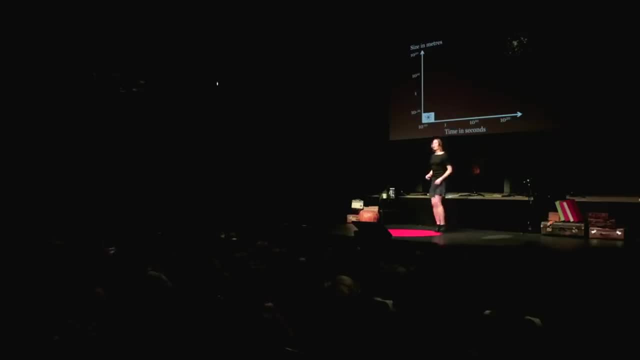 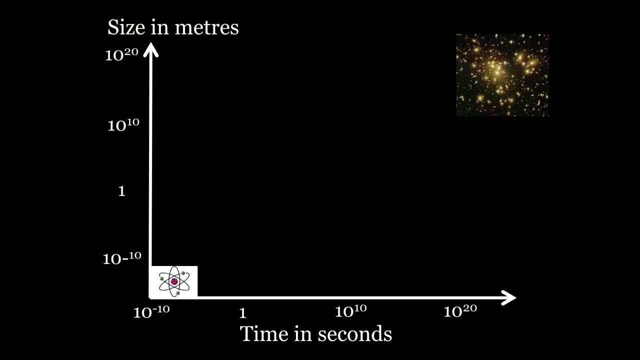 bottom, big things up there. So our current cultural image of physics looks like this: There's quantum mechanics down in that corner. It's very small, It's very weird, It happens very quickly And it's a long way down in the general, you know, on the scale of anything that matters for everyday life. And 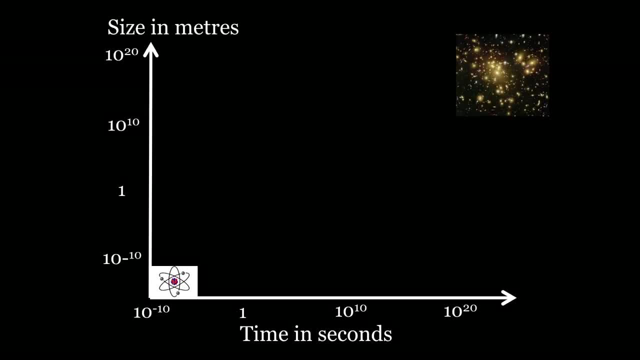 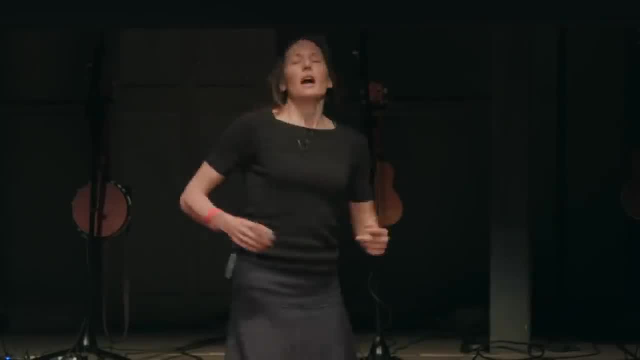 then there's cosmology, which is up there, very large, very far away, also very weird, And if you go to some places like black holes in the beginning of the universe, those two join up around the back And we know that these are frontiers in physics. right, There's lots of work being done to discover. 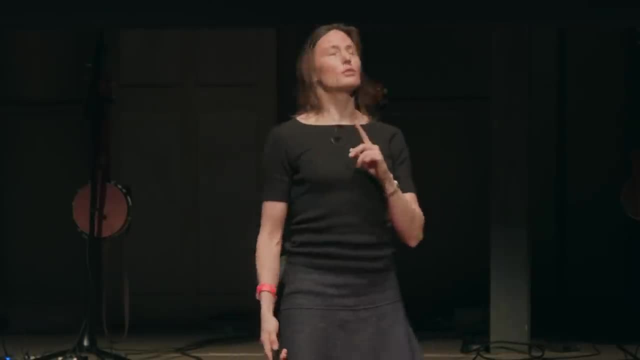 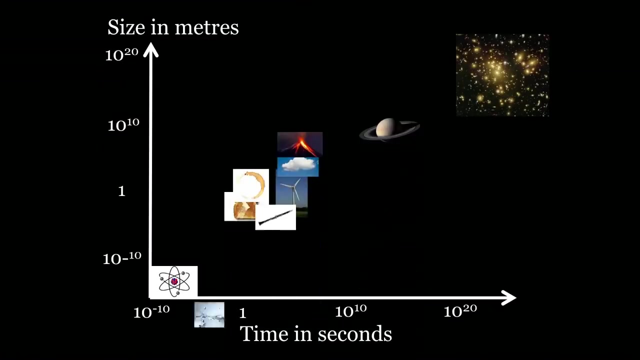 new physics in these places. But the thing is, you will notice, there's a very large gap in the middle And in that gap there are many things. There are planets and totes, and volcanoes, and clouds, and clarinets, and bubbles, and dolphins and all sorts of things that make up our everyday life. 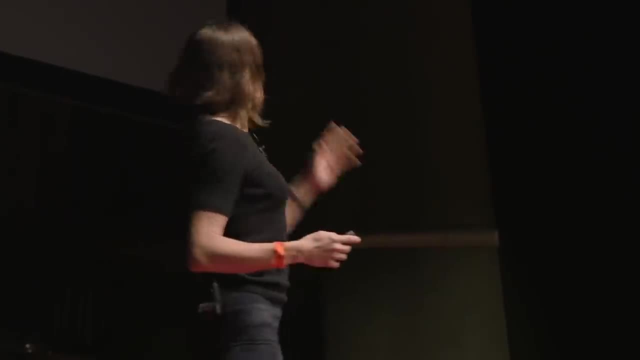 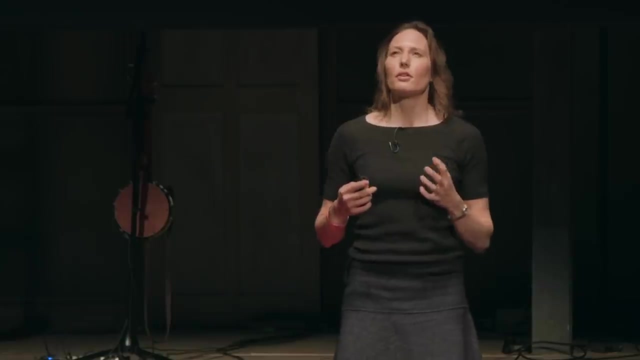 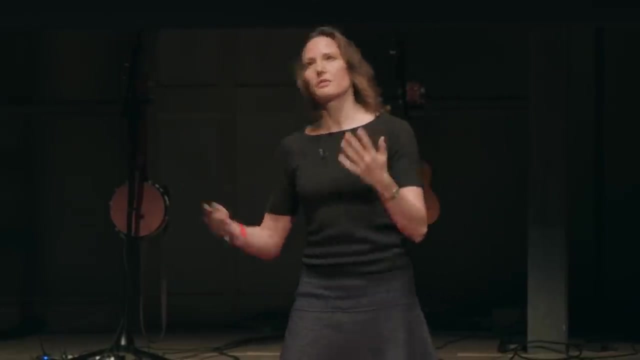 And these are also run by physics. You'd be surprised There is physics in the middle, It's just nobody talks about it. And the thing about all of these is that they all run on some relatively small number of physical laws, things like Newton's laws of motion, thermodynamics, some. 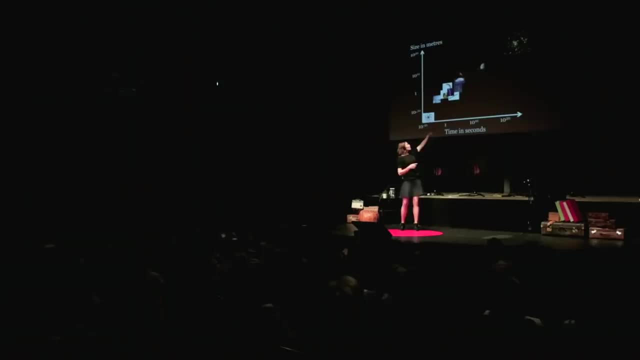 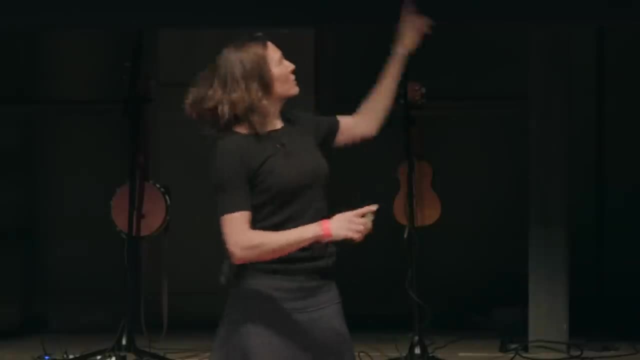 rotational dynamics. The physics in the middle applies over a huge range from very, very small things to very, very big things. You have to try very hard to get outside of this, And there is also a frontier in research physics here. It's just that nobody talks about it, And this is the world. 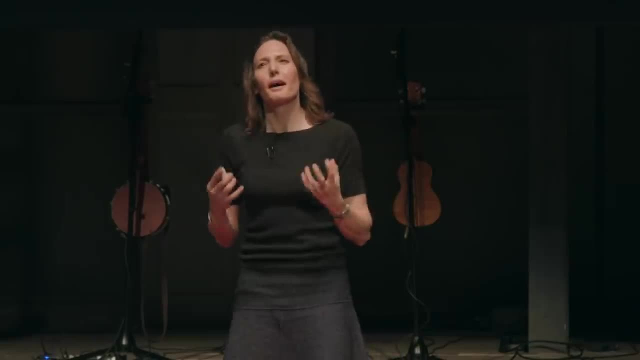 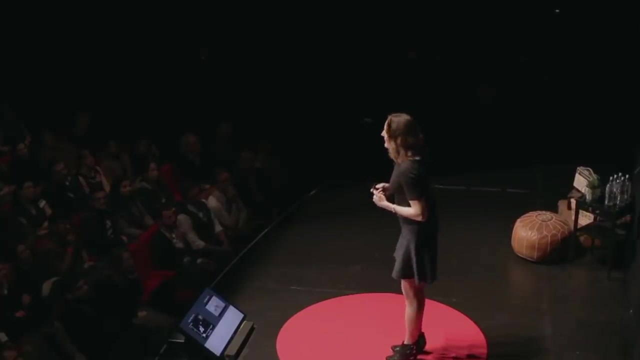 of the complex And these laws work together. They bring about the beautiful, messy, complex world we live in And, fundamentally, this is the bit that really matters to me on an everyday basis And this is the bit that we don't talk about. There's plenty of physics research going on here, But because it 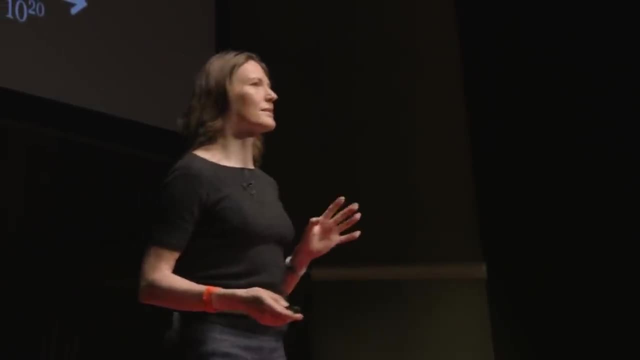 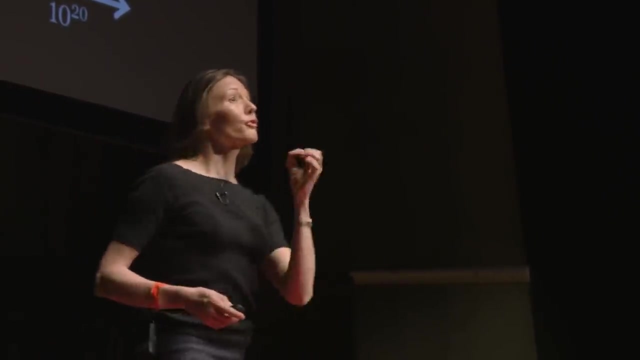 doesn't involve pointing at stars. people somehow, for some reason, think it's not there. Now, the cool thing about this is that there's so many things in this middle bit all following the same physical laws, that we can see those laws at work. 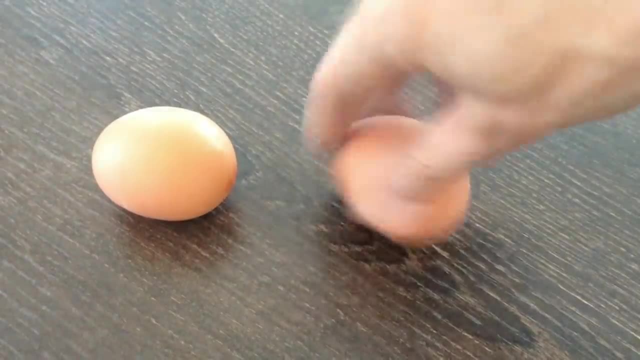 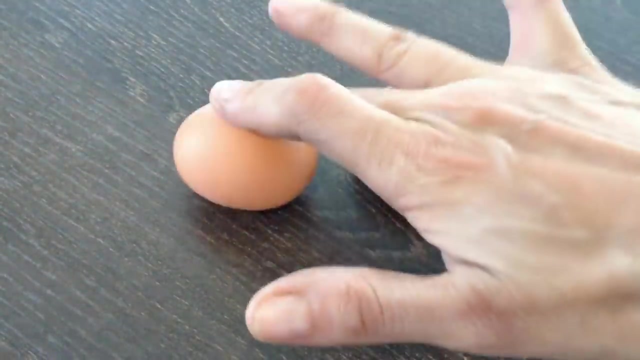 Almost all the time around us, So I've got a little video here. So the game is: one of these eggs is raw and one of them has been boiled, And I want you to tell me which one's which. It's good, that isn't it? 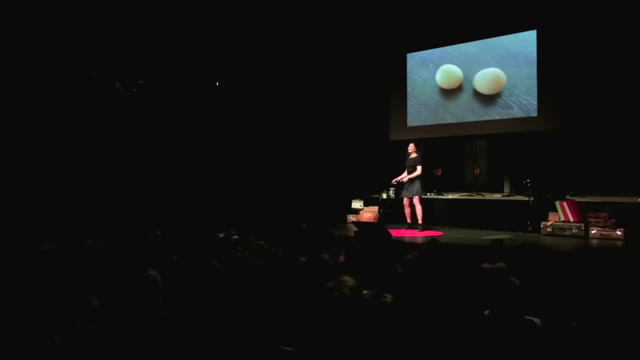 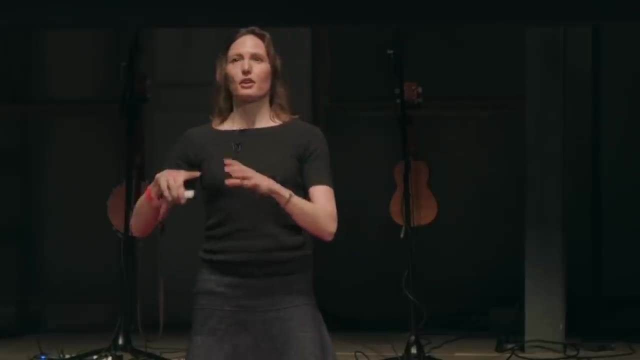 Which one's raw? The one on the left? Yes, And even though you might not have tried, that you all knew, And the reason for it is that you set the spinning. That's all right. And then, when you stop the cooked, 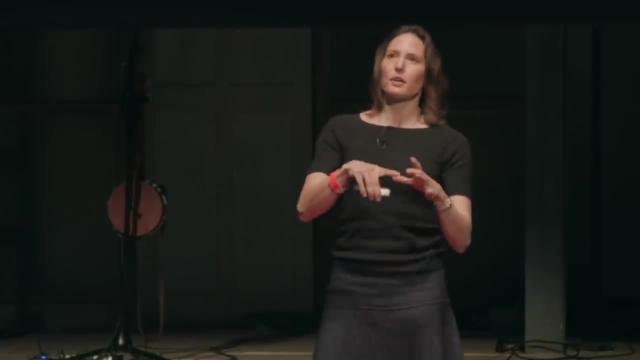 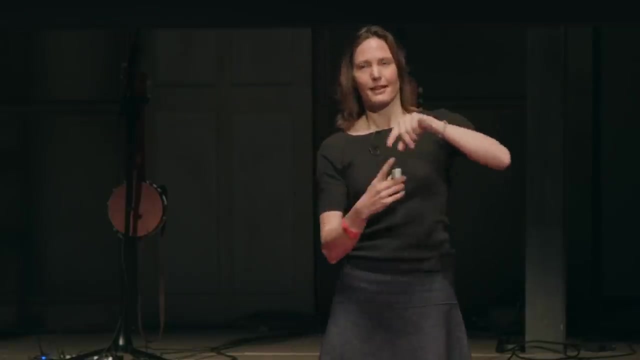 egg, the one that's completely solid, you stop the entire egg. When you stop the other one, you only stop the shell. The liquid inside is still rotating, nothing's made it stop, and then it pushes the shell around again so that the egg starts to. 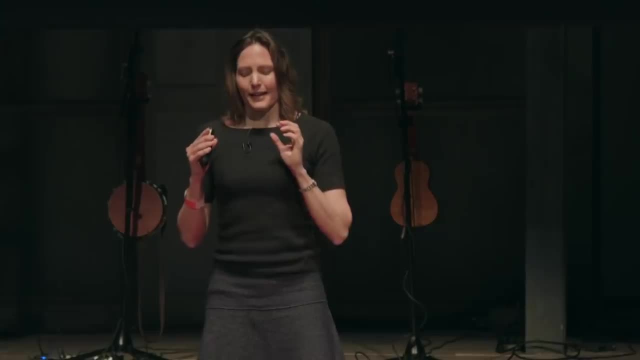 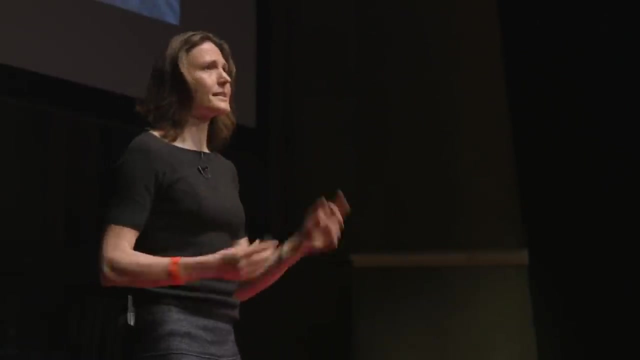 rotate again, and this is brilliant, right? uh, it's a demonstration of something in physics that we call the law of conservation of angular momentum, which basically says that if you set something spinning about a fixed axis, it will keep spinning unless you do something to stop it, and that's. 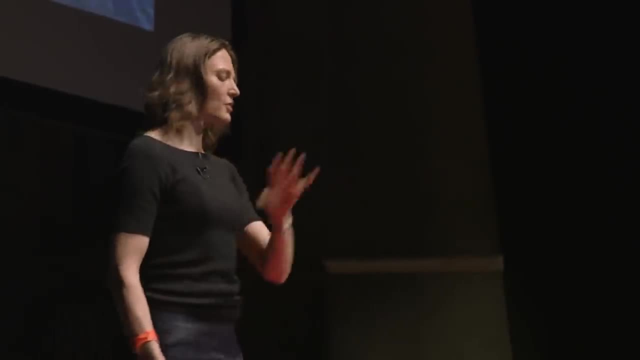 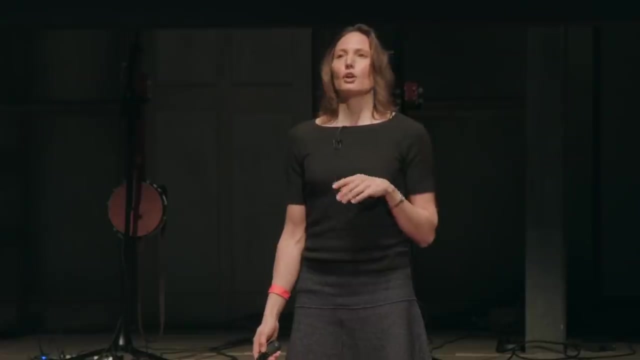 really fundamental, uh, in how the universe works, and it's not just eggs that it applies to, although it's really useful. if you're the sort of person- and apparently these people do exist- who boil eggs and then put them back in the fridge, who does that? don't admit to it, it's okay, we won't judge. 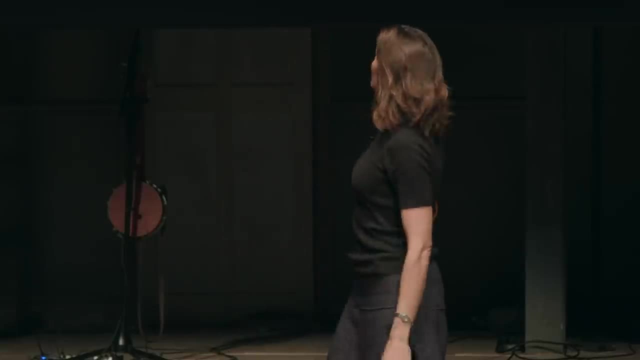 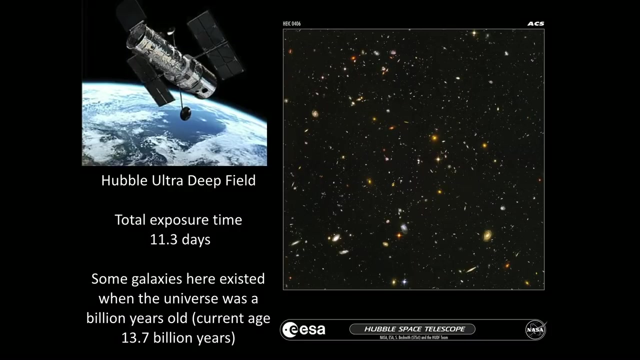 you um so, but it's also got much broader applicability. so this is the hubble space telescope, the hubble ultra deep field, which is a very tiny part of the sky, and hubble has been floating in free space for 25 years not touching anything, and yet it can point to a tiny region of 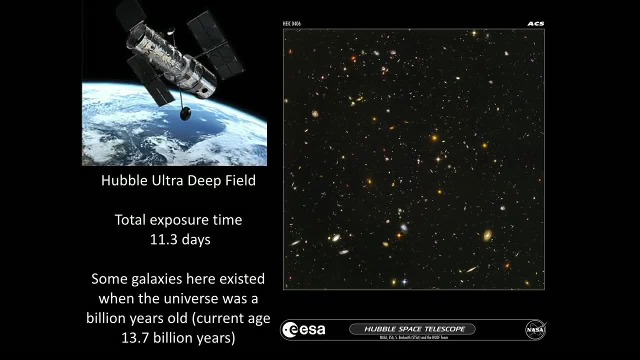 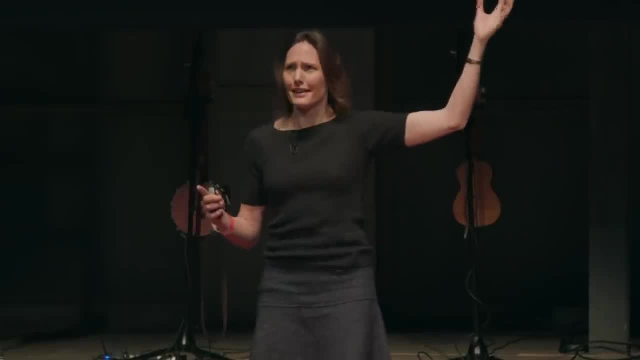 sky for 11 and a half days. it did it in sections um, accurately enough to take amazing images like this. so the question is: how does something that is not touching anything, how does it know where it is? and the answer is that in the middle of it. it has something that, to my great disappointment, isn't a raw egg but basically does the same job. it's got gyroscopes which are spinning and because of the law of conservation of angular momentum they keep spinning with the same axis, uh, indefinitely, and hubble kind of rotates around. 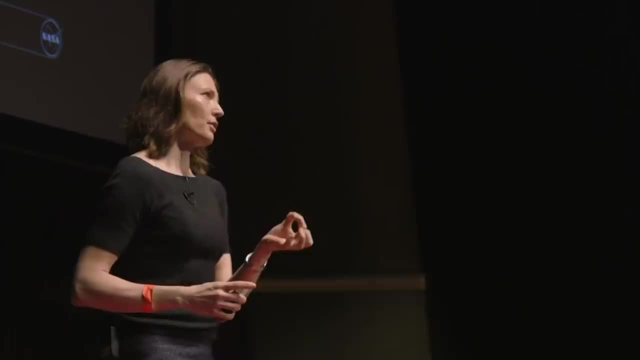 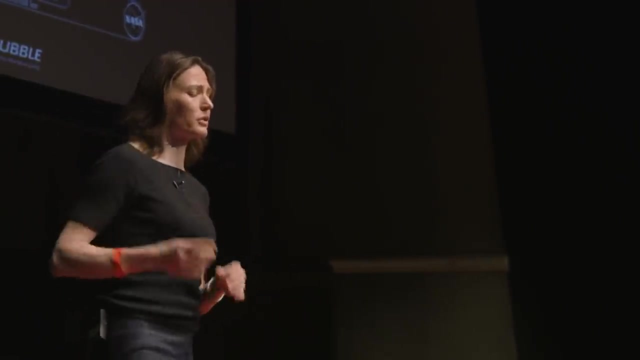 them, and so it can orient itself. so the same little physical law that we can play with in the kitchen and use also explains some of the what makes possible some of the most advanced technology of our time. and so you start. so this is the fun bit of physics: for me, it's that you learn these patterns and then 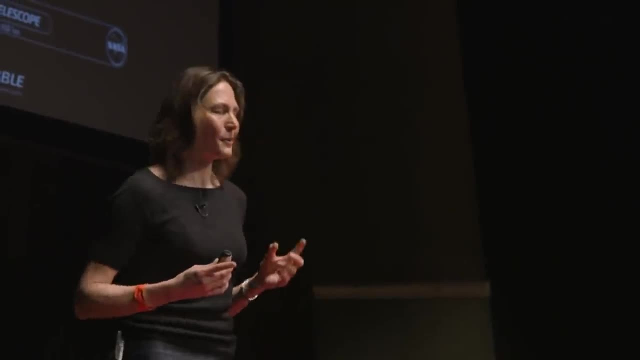 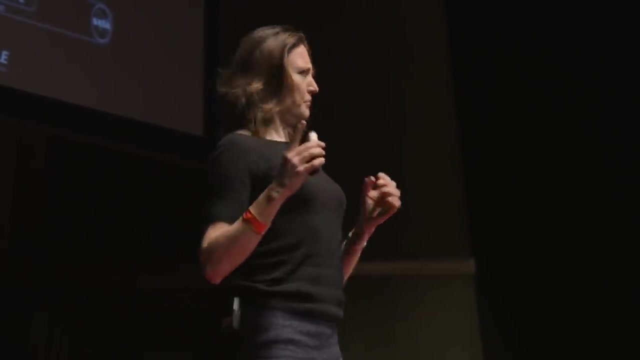 you can apply them again and again and again and it's really rewarding, uh, when you spot them in new places. this is the fun of physics. i have shown that egg video um to a an audience full of business people once, and they're all very sort of dressed up very smartly and trying to employ. 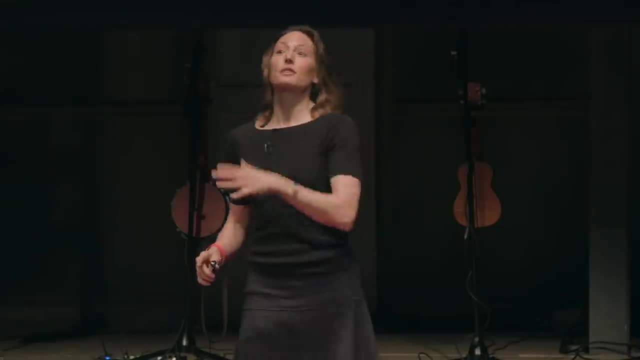 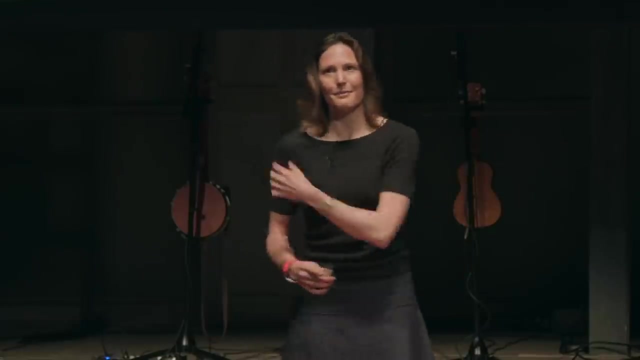 that trying to impress their bosses. and, um, i ran, it was really out of time, so i showed the egg video. you can work it out. you can ask me afterwards to check. uh, and i left the stage and then i had literally middle-aged, grown men tugging on my sleeve afterwards saying: is it this? is it this? 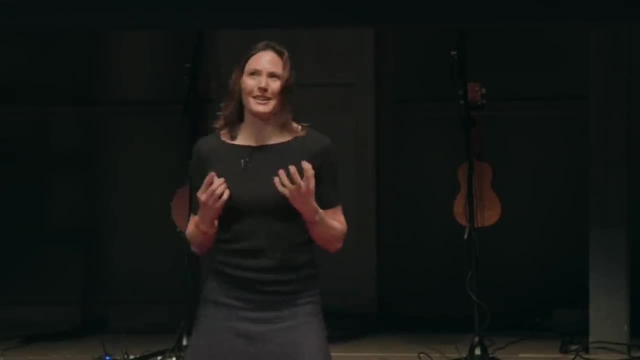 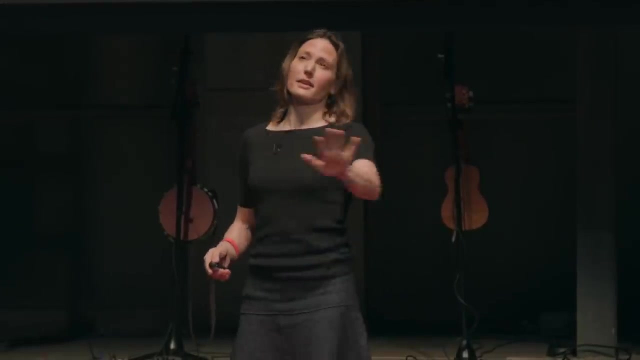 and then i said, yes, they were, yes, right. the joy that you get from like these, spotting these patterns, doesn't go away when you're an adult. and that's really important, because physics is all about patterns, and the small number of patterns give you access to all- almost all, of the physics. 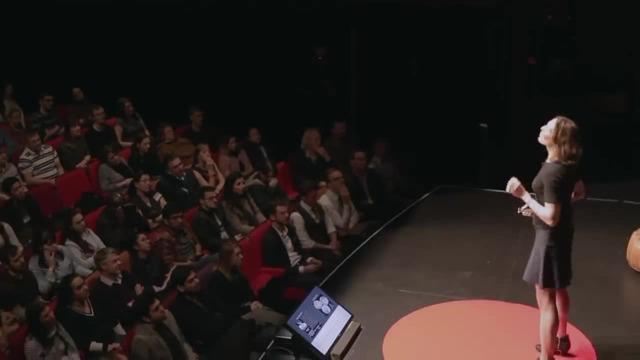 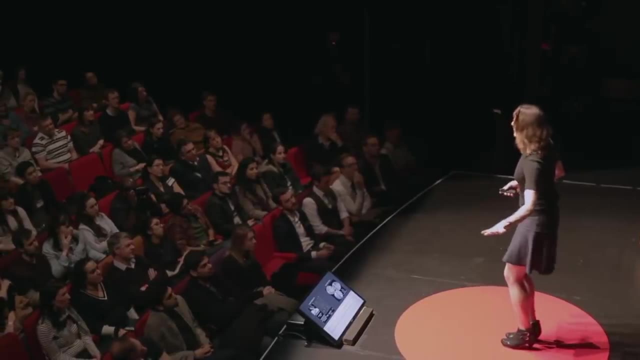 in our everyday world, and the thing that's best about this is it involves a lot of different patterns and it involves playing with toys. things like the egg shouldn't be dismissed as the mundane little things that we just give the kids to play with on a saturday afternoon to keep them quiet. 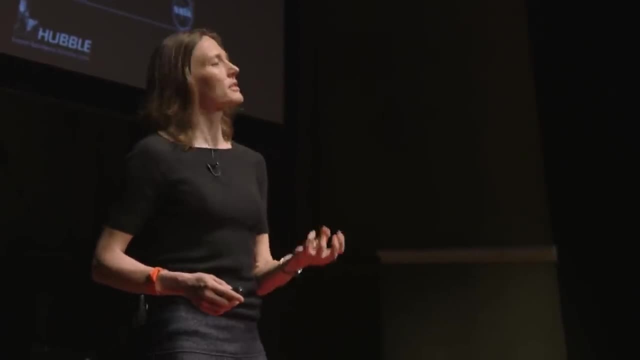 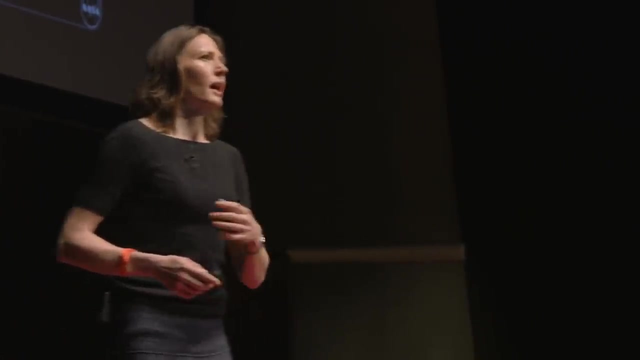 this is the stuff that actually really matters, because this is the laws of the universe and it applies to eggs and toast, falling butter side down and all sorts of other things, just as much as it applies to modern technology, um, and anything else that's going on in the world. so i think we 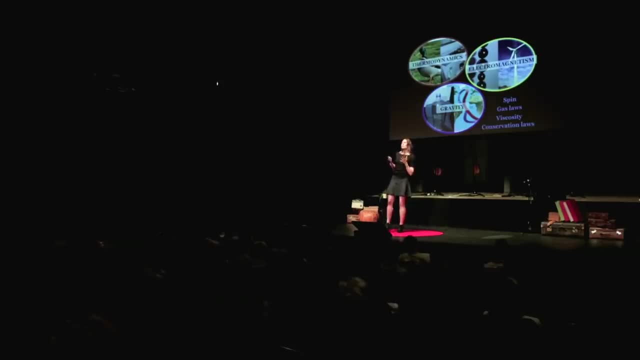 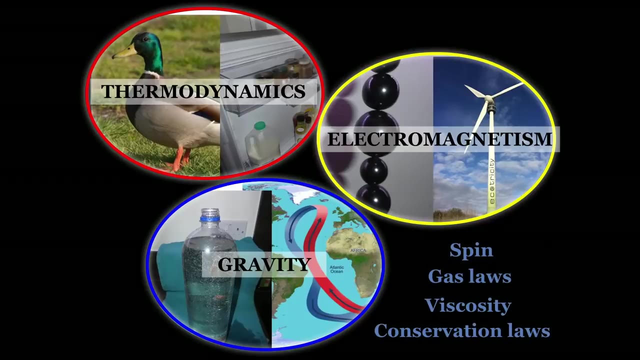 should play with these patterns. so there are- basically there are a small number of concepts that you can become familiar with using things in your kitchen that are really useful for life in the outside world. if you want to learn about thermodynamics, a duck is a good place to start, for example. 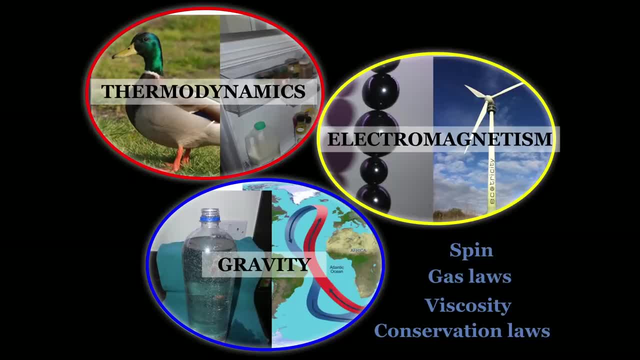 why their feet don't get cold. and once you've got a bit of thermodynamics with the duck, you can also explain fridges and magnets that you can play with in your kitchen, get you to wind turbines and modern energy generation. um raisins in lemonade, which is always a good thing to play with if 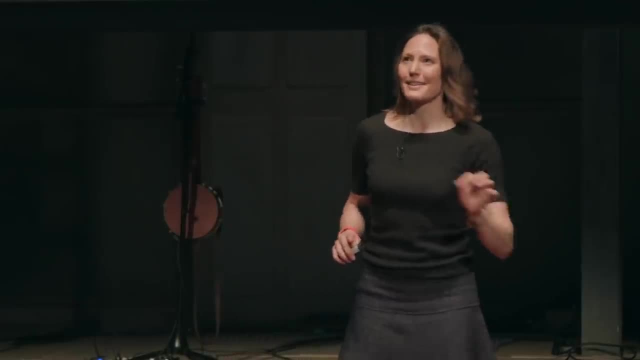 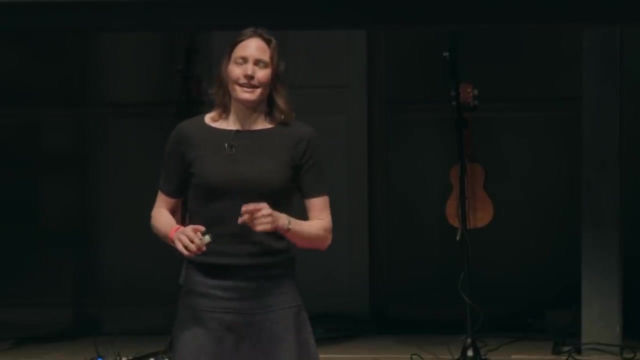 you're at a boring party, fish some raisins out of the bar snacks, put them in some lemonade. uh, it's got three consequences. first thing is: it's quite good to watch, try it. secondly, it sends the boring people away. thirdly, it brings the interesting people to you. you win on all fronts. um and then. 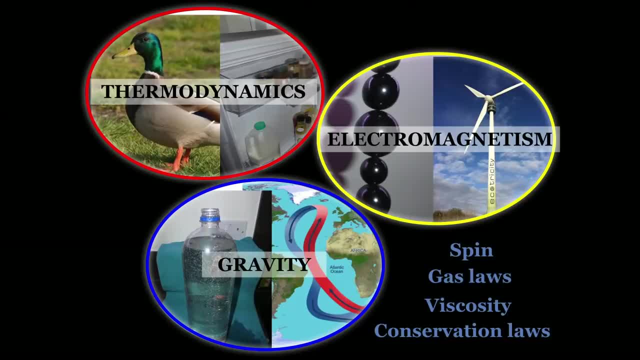 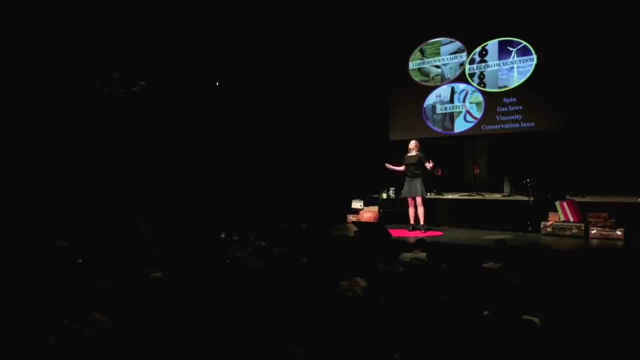 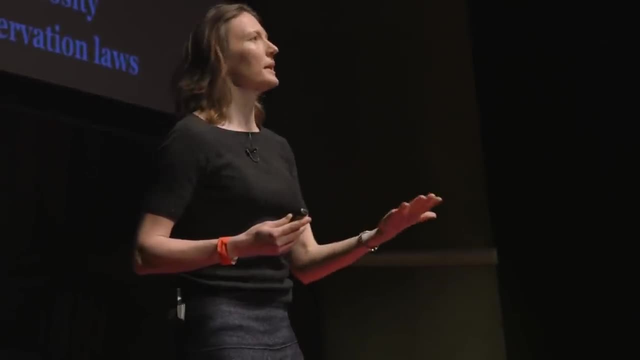 there's. there's things you know: spin and gas, laws and viscosity. there's these little patterns and they are right around us everywhere and it's fundamentally democratic right. everybody has access to the same physics. you don't need a big posh lab. when i- um, when i wrote the book and i i had the chapter on spin and i'd written a bit about toast. 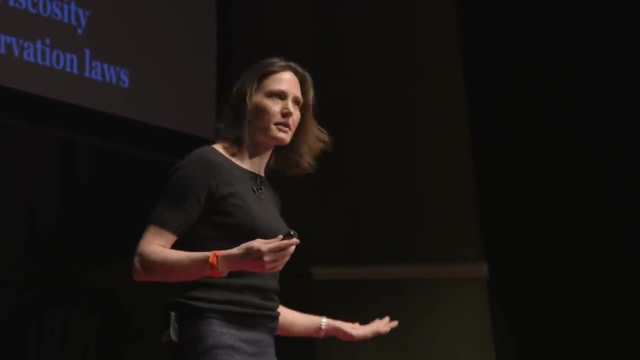 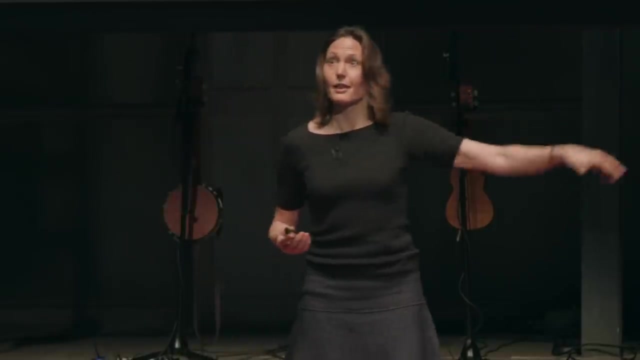 butterside down and i gave the chapter to a friend of mine who's not a scientist and for him to read: tell me what you thought. and he took the um, took the chapter away and he was working overseas and i got this text message back from him a couple of weeks later and it said: um, i'm at breakfast in a 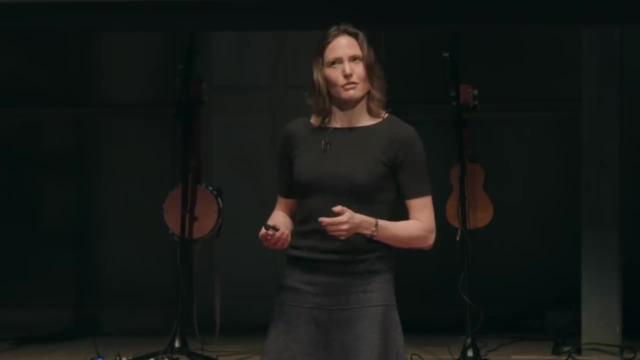 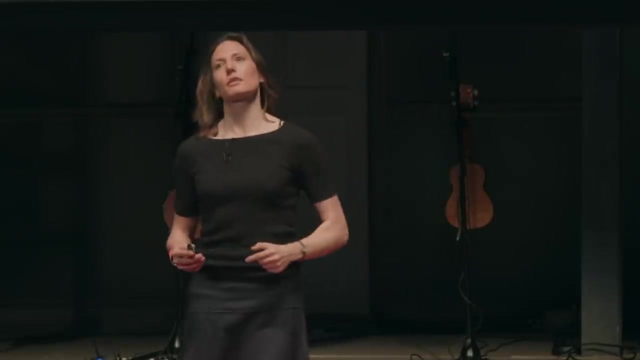 posh hotel in switzerland and i really want to push toast off the table because i don't believe what you wrote. and that was the good bit. he doesn't have to. he can push the toast off the table and that's the thing about science. and science is that it's not about the science. right, there's. 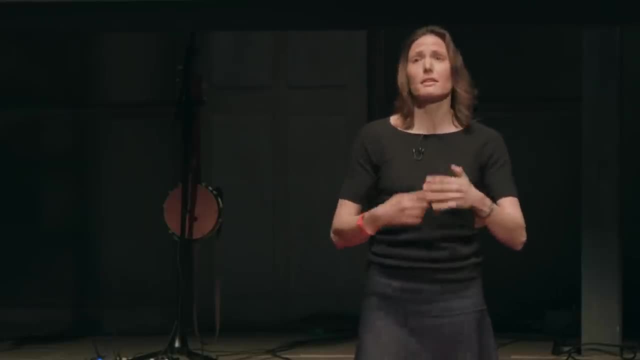 the fundamental laws that we have learned through experience and experimentation work right the day we drop an apple and it goes up. then we'll have a debate about gravity. up to that point, we basically know how gravity works and we can learn the framework, and then it's the process of 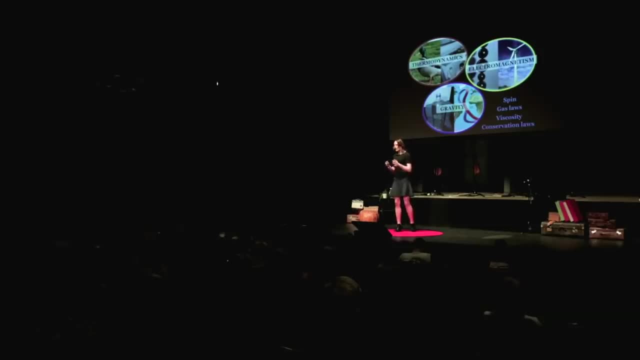 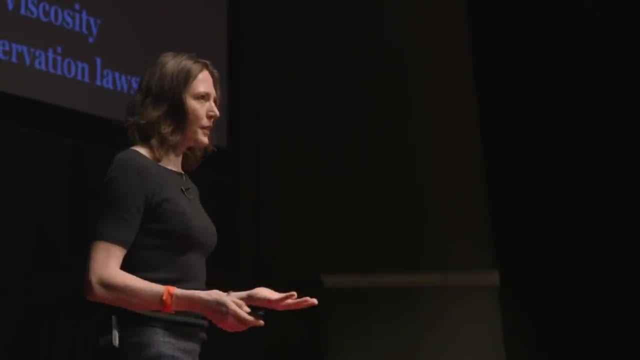 experimentation, having confidence in things, trying things out, critical thinking, how we move science forward, and you can learn both of those things by playing with toys in the everyday world. um, and it's really important because, you know, there's all this talk about technology we've heard talks about 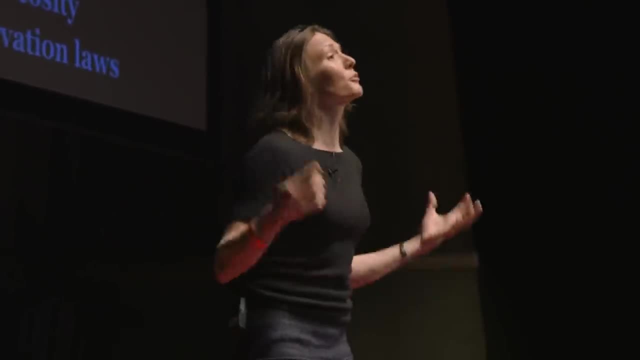 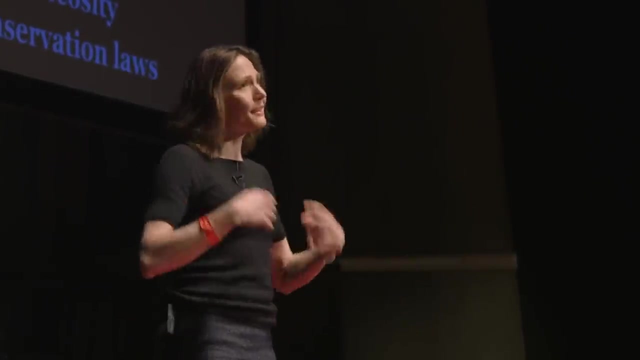 quantum computing and all these sort of mysterious, far-off things. but fundamentally, we still live in bodies that are about this size. we still walk about, sit on chairs that are about this size. we still live in the physical world and knowing being familiar with these concepts means we're not. 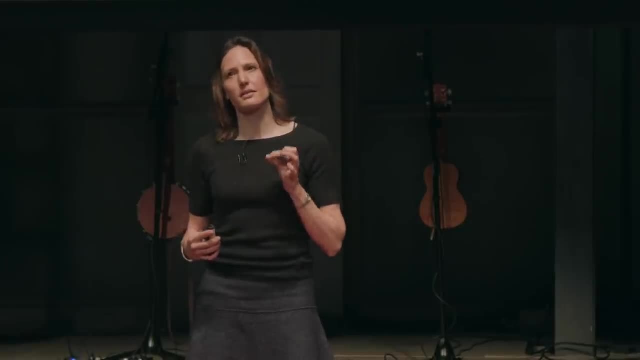 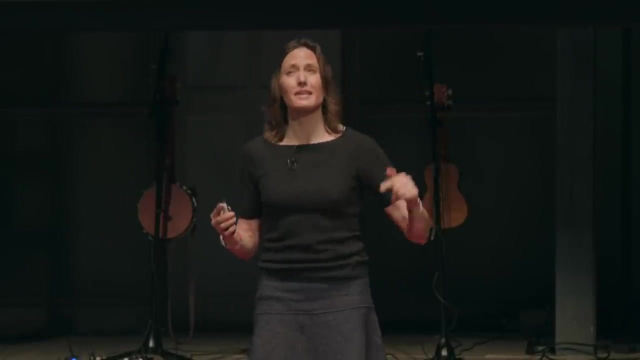 helpless, and i think it's really important that we're not helpless, that society feels it can look at things, because this isn't about knowing all the answers. it's about having the frameworks you can, the right questions, and by playing with these fundamental little things in everyday life, we 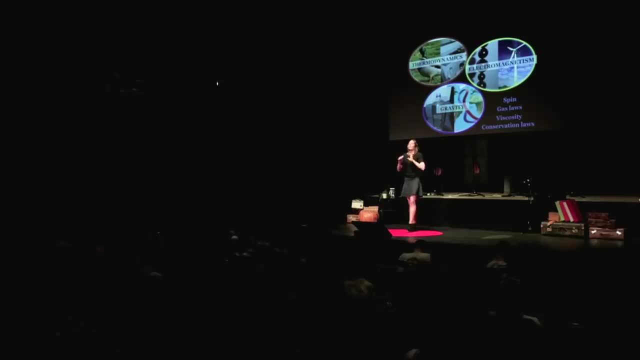 gain the confidence to ask the right questions. so there's a bigger thing. um, in answer to nana's question about what you can do when you know that, because there's lots of stuff in the everyday world that you can do when you know that, especially if you've got eggs in the fridge- um, and there's a 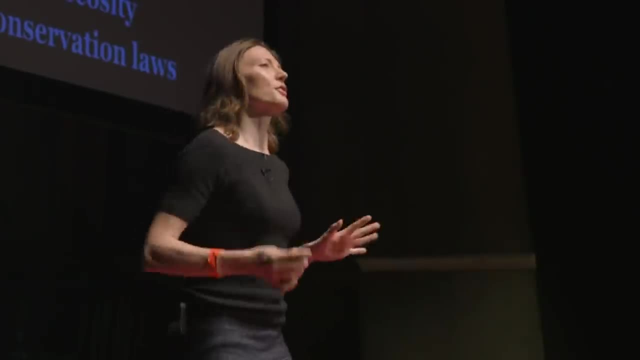 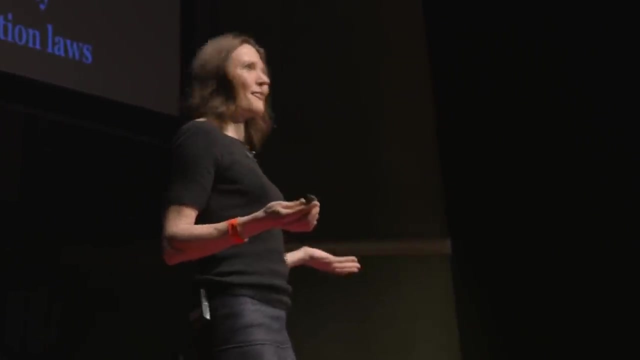 much deeper answer. uh, and so there's all the fun and the curiosity that you could have playing with toys. because we shouldn't, by the way, toys not. why should kids have all the fun? right, all of us can have fun playing with toys and we shouldn't be embarrassed about it. you can blame me, it's fine. 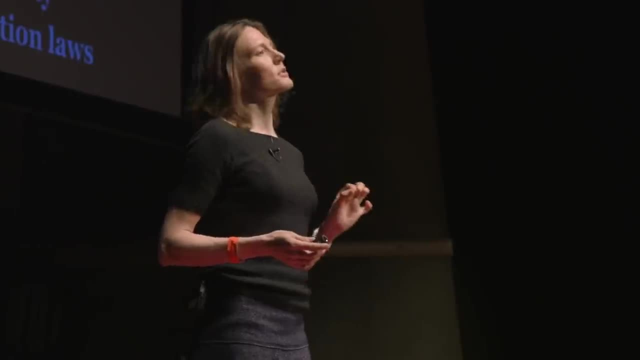 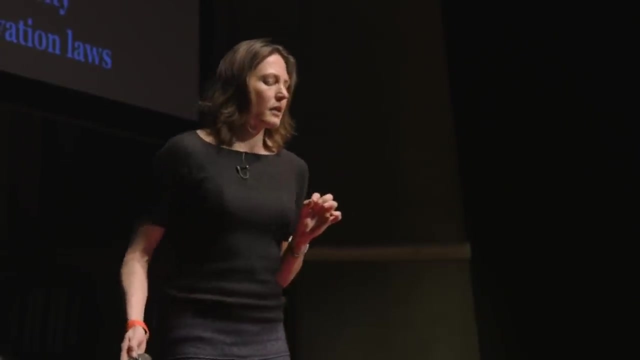 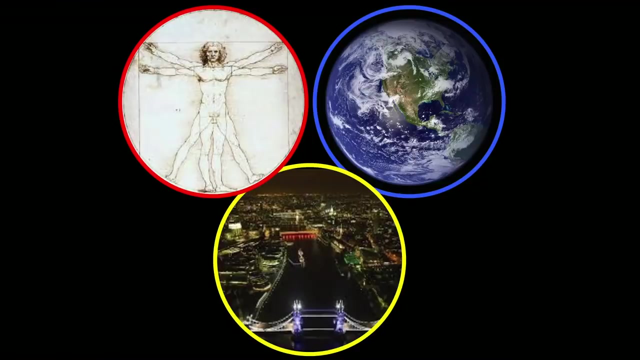 um. so when it comes to reasons for studying physics, for example, here is the best reason i can think of. i think that each of us has three life support systems. we've got our own body, we've got a planet and we've got our civilization. each of those is an independent life support. 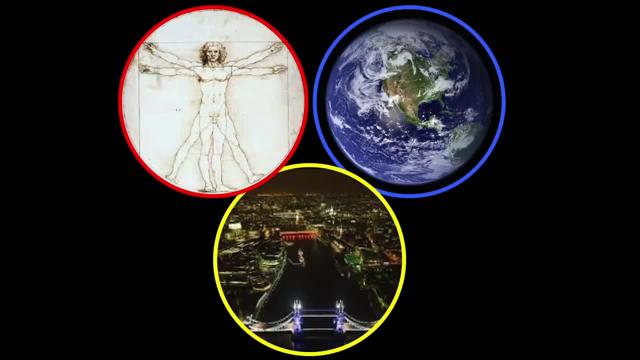 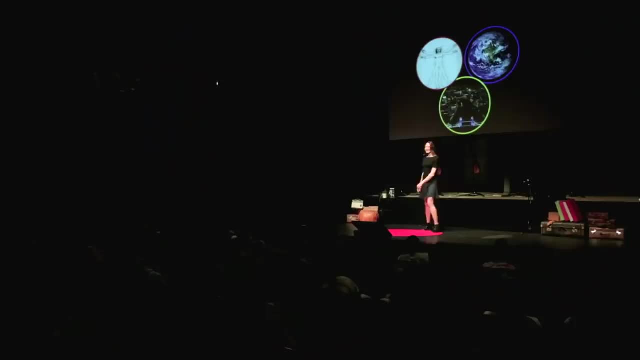 system keeping us alive in its own way, and they all run on the fundamental physical laws that you can learn in the kitchen with eggs and teacups and lemonade and everything else you can play with. So this is the reason, for example, that something like climate change is such a serious problem. it's because it's 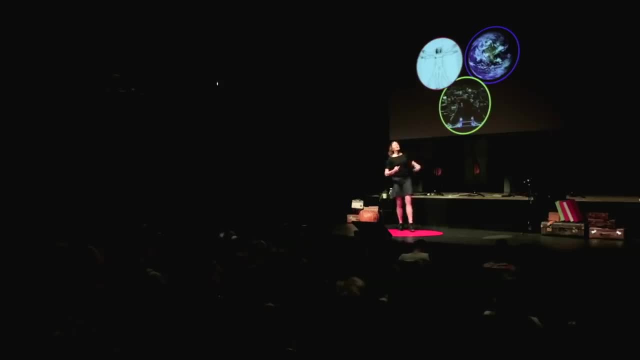 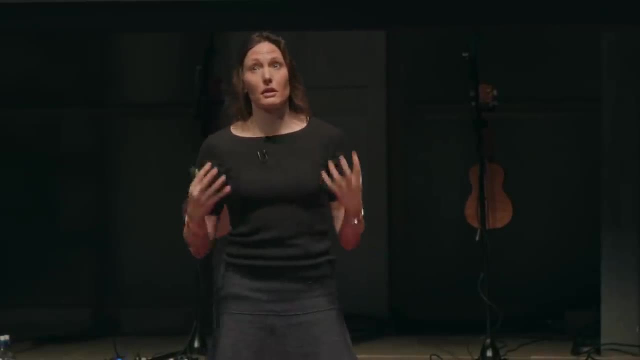 two of these life support systems, our planet and our civilization, kind of butting up against each other. they're in conflict and we need to negotiate that boundary. and the fundamental physical laws that we can learn, that are the way the world around us works, are the tools at the basis of 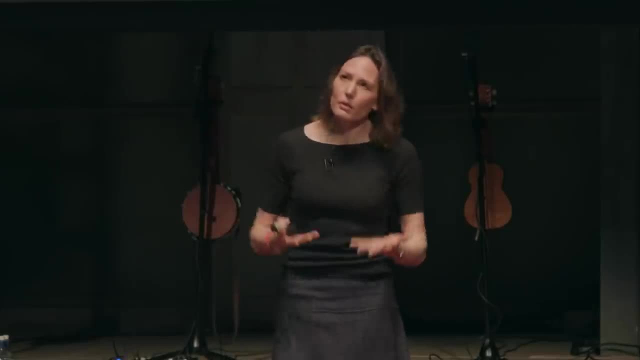 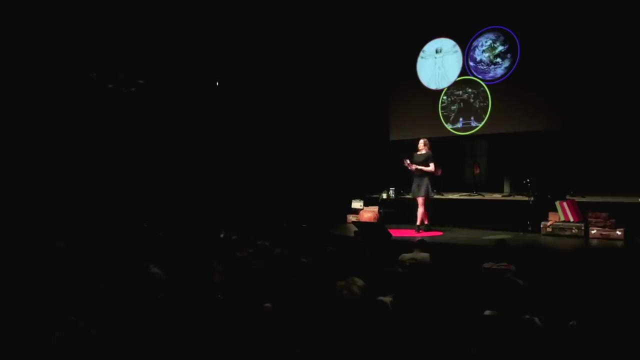 everything. they're the foundation. there's lots of things to know about in life, but knowing the foundations is going to get you a long, long way, and I think this, if you're not interested in having fun with physics or anything like that, strange, but anyway, apparently these people exist and you can. 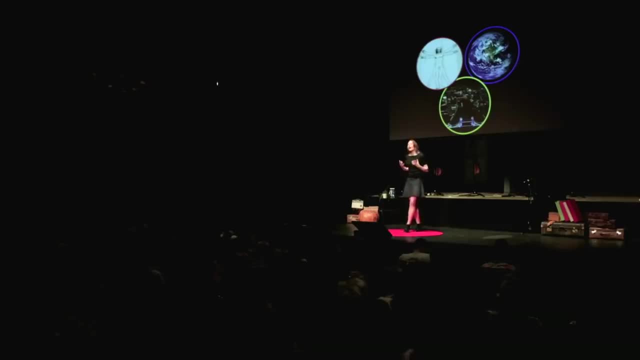 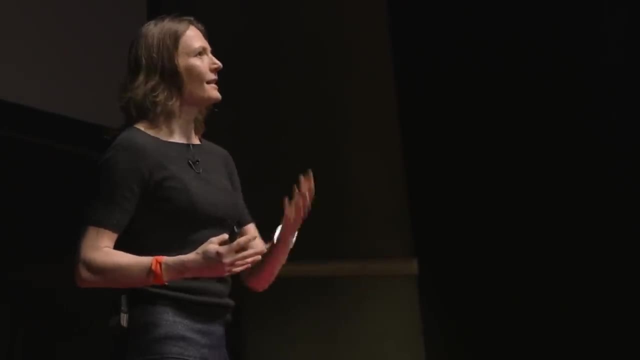 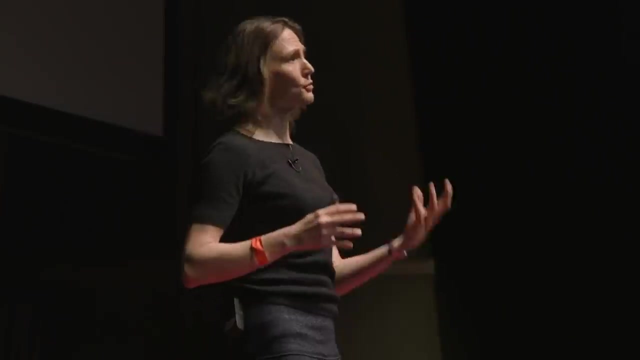 you surely are interested in keeping yourself alive. right, and how our life support systems work, because the framework for physics is remarkably constant. Right, it's the same in lots and lots of things that we measure. it's not going to change anytime soon. they might discover some new quantum mechanics, but apples right here are still going to fall down. 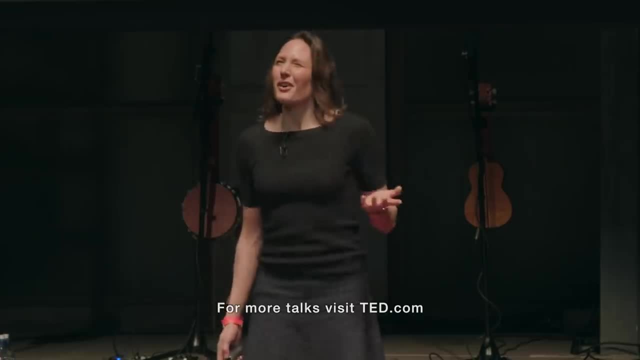 so the question is how I got asked. you know, I get asked sometimes: how do you start? what's the place to start if you're interested in the physical world, in not being helpless and in finding some toys to play with? So here is my suggestion to you. so some things to start with, so it starts right. 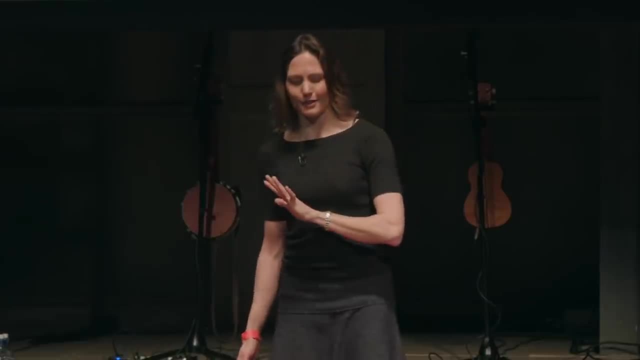 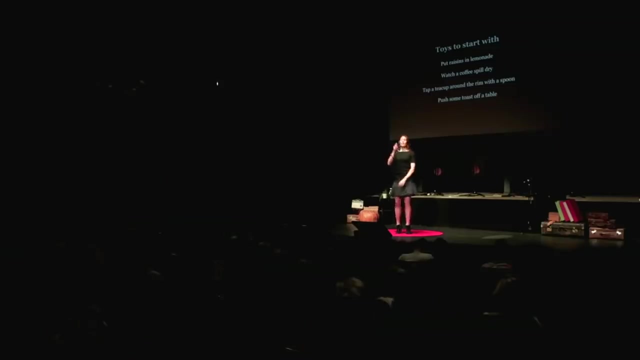 the place that starts is that moment. and adults do this. right, you, you're drifting along somewhere and you spot something and your brain goes, oh, that's weird. and then your conscious nose goes: oh, you're an adult, keep going. and I- that's the point right, hold that thought that. 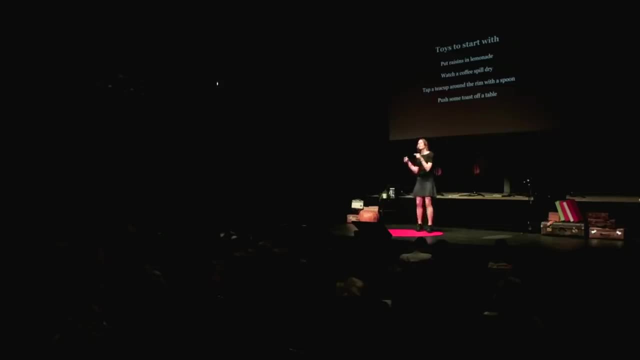 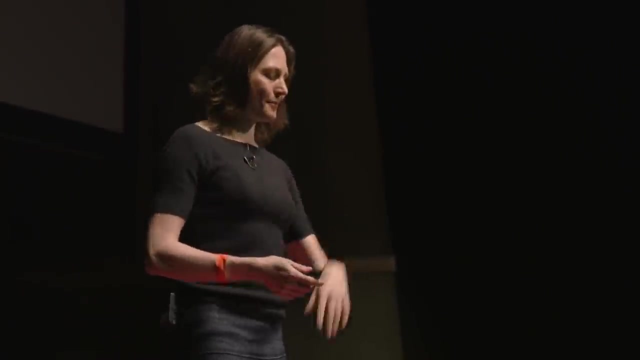 bit where your brain went. oh, that's a bit odd, because there's something there to play with and it's worth you playing with it. so that's the place to start, but if you don't have any of those little moments, uh, on your way home from from this event, here are some things to start with. like I said, put. 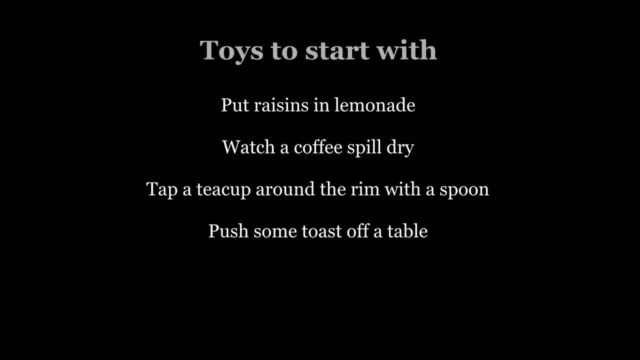 raisins and lemonade. it's highly entertaining. um, watch your coffee spill dry. I know that sounds a little bit weird, but it's a little bit weird, and it's a little bit weird. and it's a little bit weird like watching paint dry, uh, but it does do quite weird things. it's worth watching. um get, I am you. 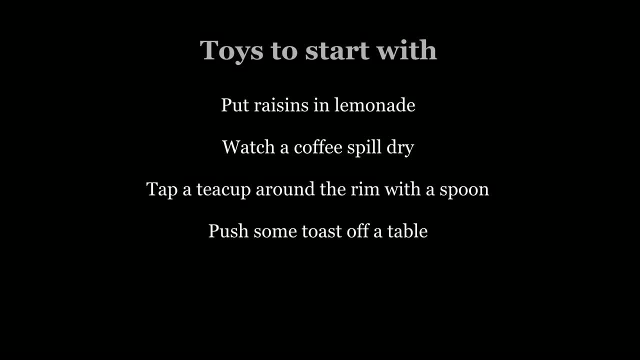 know what I'm an acquired taste at dinner parties if there are teacups around. there are so many things you can do to play with teacups. it's brilliant. uh, the most obvious one is to get a teacup. get a spoon, tap the teacup around the rim and listen, and you will hear something strange. 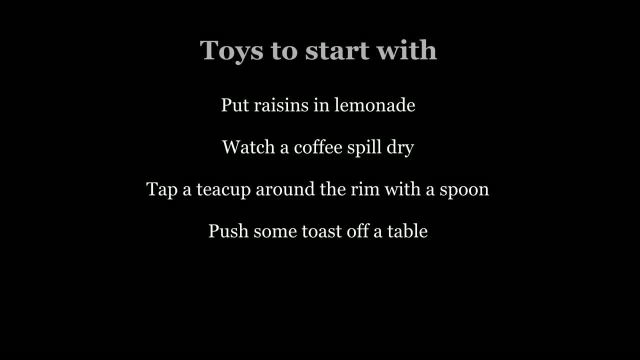 uh, and the other thing is: push a toast off the table. push some toast off the table because you can right and you'll learn stuff from it. and if you're feeling really ambitious, try and push it off in such a way that it doesn't hurt you and it doesn't hurt you and it doesn't hurt you. 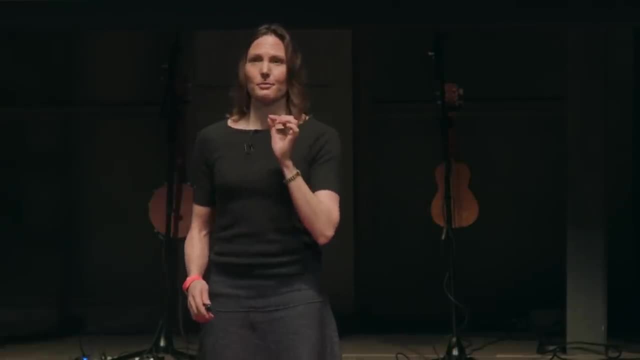 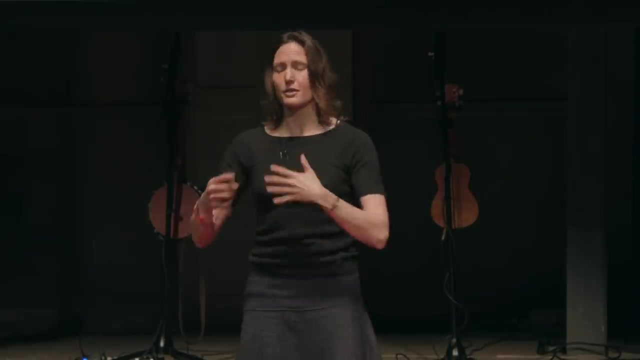 doesn't fall, but a side down, um, which is possible. so the point of all of this is that, first of all, we should all play with toys, right? we shouldn't be afraid to investigate the physical world for ourselves with the tools around us, because we all have access to them. it matters because if we want 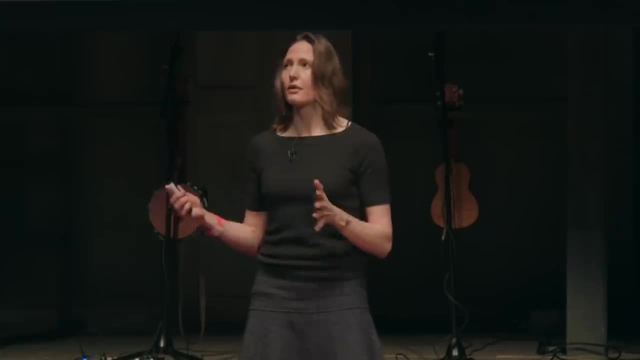 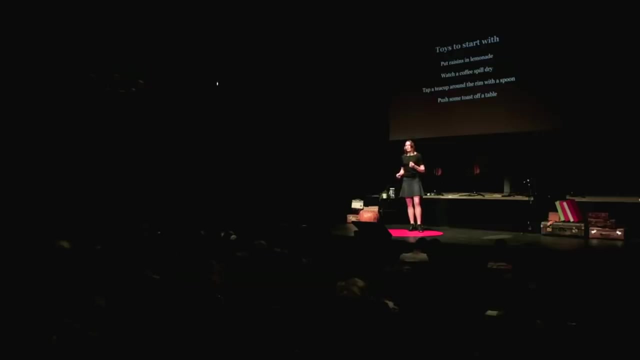 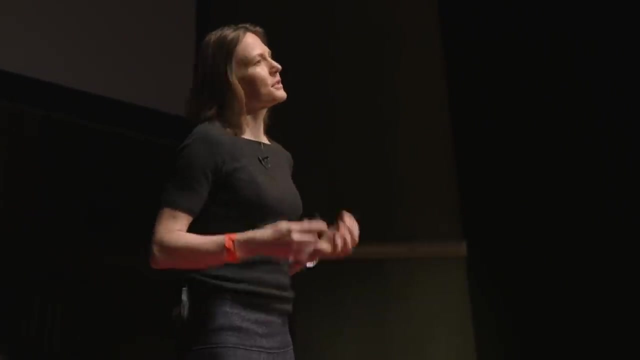 to understand society. if we want to be good citizens, we need to understand the framework on which everything else must be based. so playing with toys is great, understanding how to keep our life support systems going is great, but fundamentally, the thing that we need to change in the way that we talk about physics is that we need to understand that physics isn't 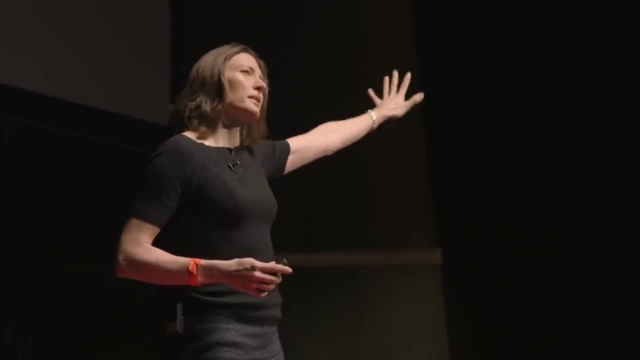 out there with weird people and strange hieroglyphics for somebody else in a posh lab. physics is right here, it's for us and we can all play with it. thank you very much. 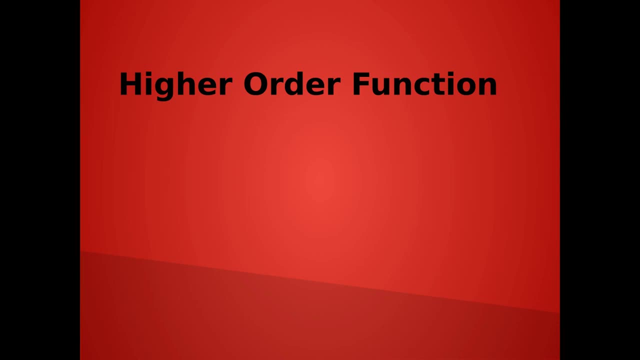 Hi, today we are going to learn what exactly the higher order functions are. So let's go to the definition. So definition of higher order function is: higher order function is a function that either takes a function as an argument or return a function. So what? 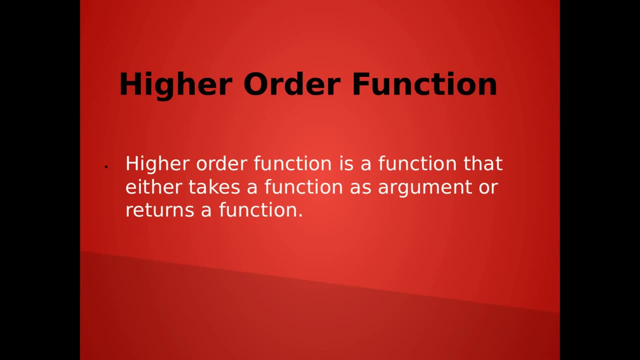 does it mean that it either takes a function as an argument or returns a function? So, as we know that whenever we create a function, we create its argument. Argument must have a data type, like it has, either have a int, double or something. So in Scala we can create: 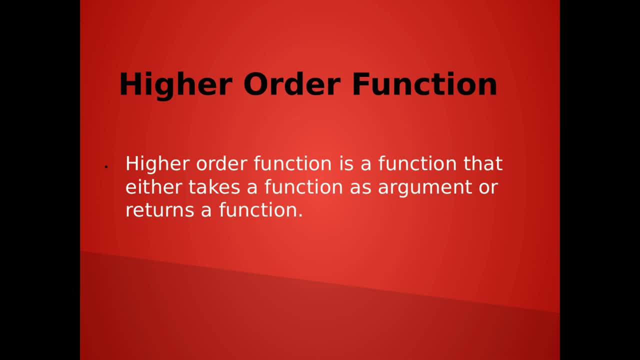